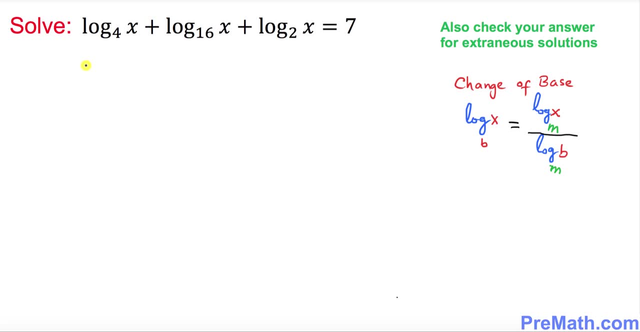 So this is going to look like this one. So you have to be a little bit careful. I'm going to put down log of x. I'm going to change to base 2.. So I'm going to put it like this one First one is log of x. 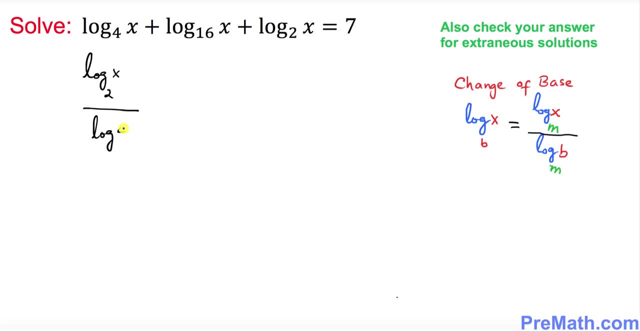 So 4 on the bottom base 2.. Likewise, plus this log of 16x with a base 16 could be written as log of x with a base 2 divided by log of 16 with a base 2.. And plus this log of x with 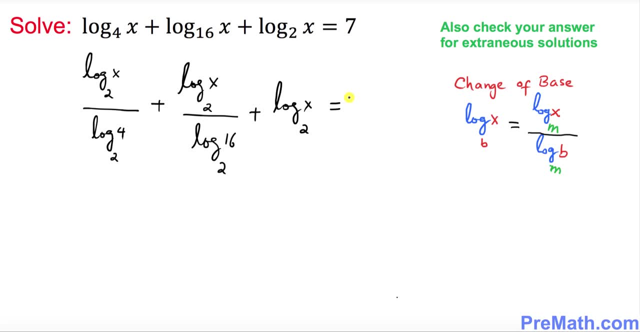 a base 2 is already there. We're just going to leave it like this, Leave it alone. And now the next thing we want to do is we want to make things simple by manipulating these numbers 4 and 16.. See how I'm going to do this thing On the top. 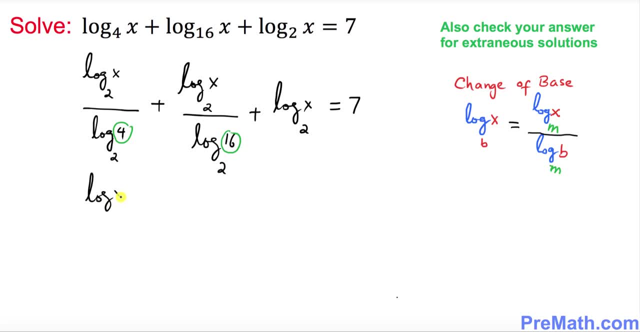 it's still going to be log of x with a base 2 divided by. I can write: log of 4 could be written as 2 power 2 with a base 2.. That means 2 power x 1 with a base 2.. is it not? 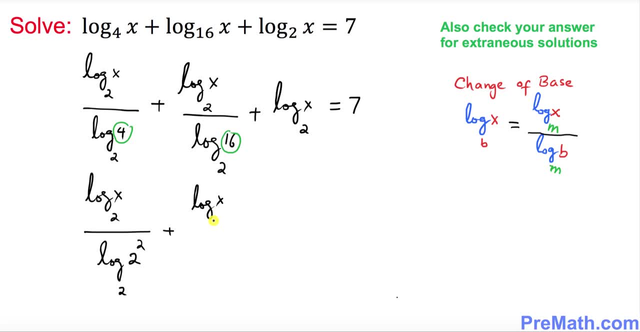 Plus numerator is same. Log of x with a base 2.. Log of x with a base 2 is equal to plus numerator is the same, And here I can write log of 16,. 16 could be written as 2 power 4 with a base 2.. 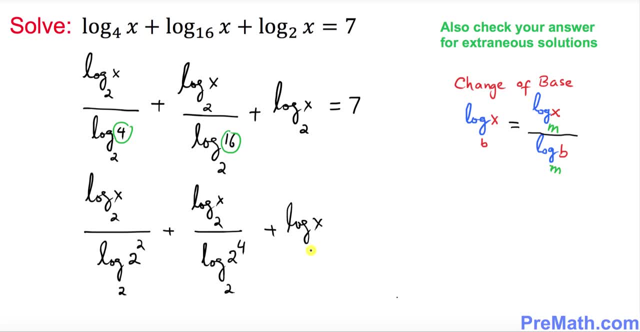 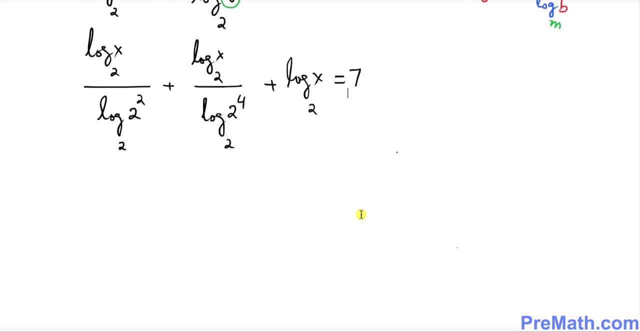 And the rest is same. So far, so good. So the next step that we'll be doing is I'm going to solve this point. So how many threes? I'm going to use big Australia. the number h is countries ihr over blijvan jurisdiction. 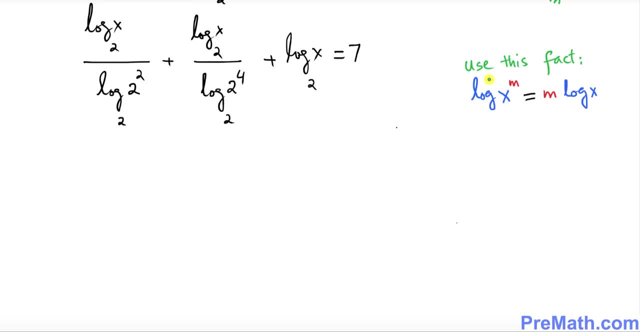 i times a number, y times a电 and v times the number and hundreds, is i times Th, and 1. and 2. will be greater or less than doing is now. we'll use this fact. if you have a log of x and you have an exponent m, then you can. 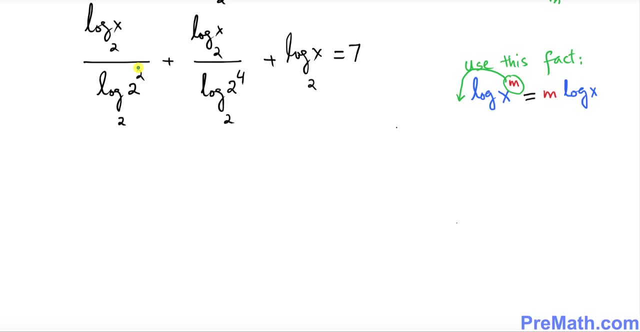 move that exponent m to the front here. in our case this is an exponent 2. we're going to move it to the front over here. likewise, this for this exponent: i can move it to the front. so our problem is going to look like then: log of x to the base 2 divided by once. you move 2 over here, so this become log of. 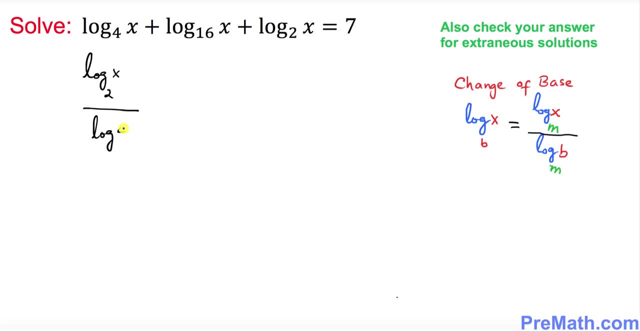 So 4 on the bottom base 2.. Likewise, plus this log of 16x with a base 16 could be written as log of x with a base 2 divided by log of 16 with a base 2.. And plus this log of x with 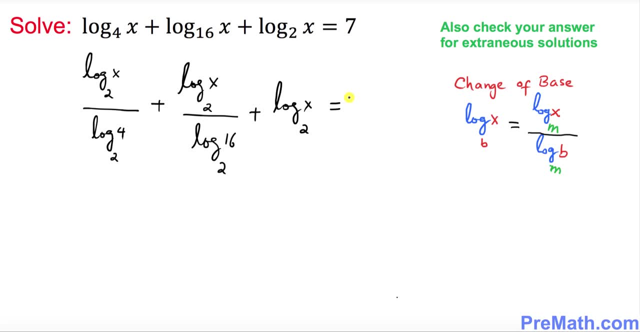 a base 2 is already there. We're just going to leave it like this, Leave it alone. And now the next thing we want to do is we want to make things simple by manipulating these numbers 4 and 16.. See how I'm going to do this thing On the top. 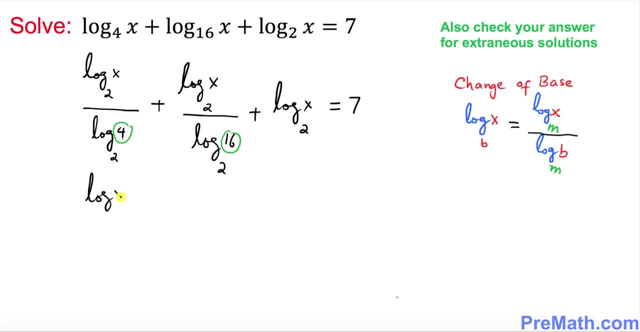 it's still going to be log of x with a base 2 divided by. I can write: log of 4 could be written as 2 power 2 with a base 2.. Yeah, So 2 power 3, plus 9x with a base 2, isn't it? 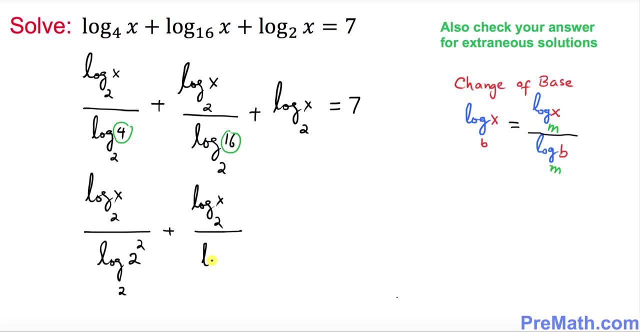 Plus numerator is same. log of x with a base 2, and here I can write log of 16.. 16 could be written as two power four with a base 2, and the rest is same. So far, so good. 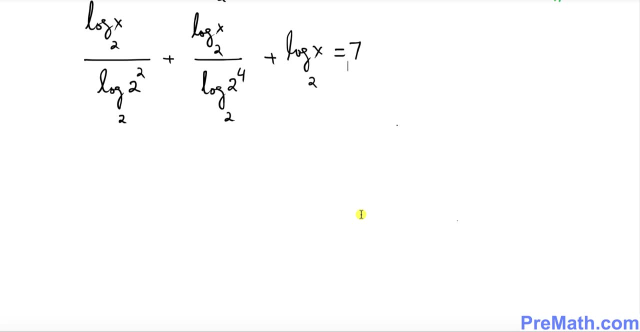 Okay, Okay, Okay, Alright, Okay, Yeah. Okay, that's what I'm going to do- is now we'll use this fact: if you have a log of x and you have an exponent m, then you can move that exponent m to the front here. in our case, this is an exponent 2. we're going to move it to the 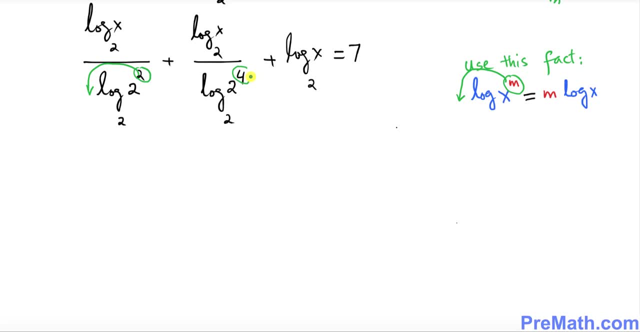 front over here. likewise this for this exponent. i can move it to the front. so our problem is going to look like then: log of x to the base 2 divided by. once you move 2 over here so this become log of 2 with the base 2 plus. log of x with the base 2 divided by 4. log of 2 with the base 2 plus. 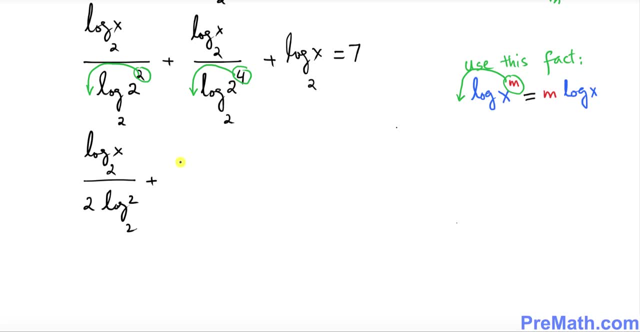 2 with the base 2 plus log of x with the base 2 divided by 4. log of 2 with the base 2 plus log of x with the base 2 equal to 7. so next thing now. I want you to just focus on this part over here. 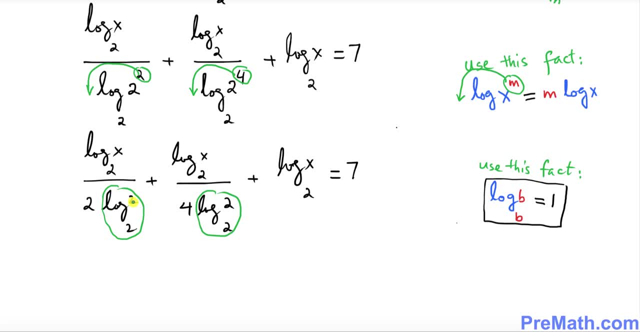 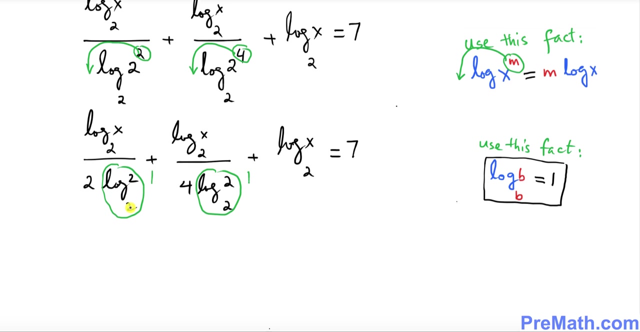 they have the, the base and the import. that's called so according to this fact, this turns out to be this. log of 2 with the base: 2 turns out to be 1, this is 1 and this is 1 as well, so our this problem could be more simplified, as you can see. log of x. 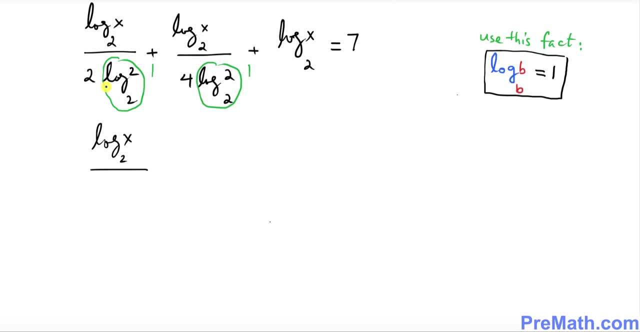 with the base 2 over 2 times 1, because this is 1, so this is simply 2 plus log of x, with the base 2 divided by 4 times 1, plus now we have a log of x with the base 2 equal to 7. so we have this fractions over here we want. 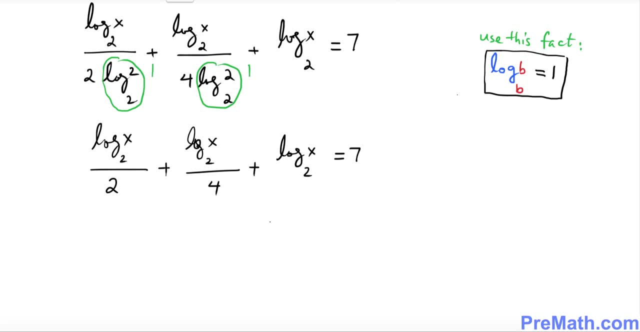 to remove them. in order to remove them, the best thing to do is I want you to multiply by that. the biggest number over here at the bottom is 4, so I'm going to multiply by 4 across the board. okay, so you do that one. so this 2 and 4 reduces to 2 times log of x with the base 2 plus this 4 and this 4 is 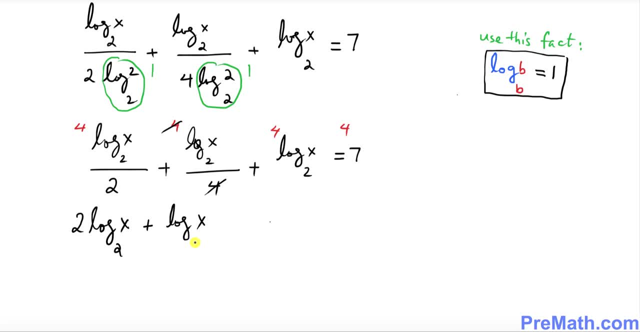 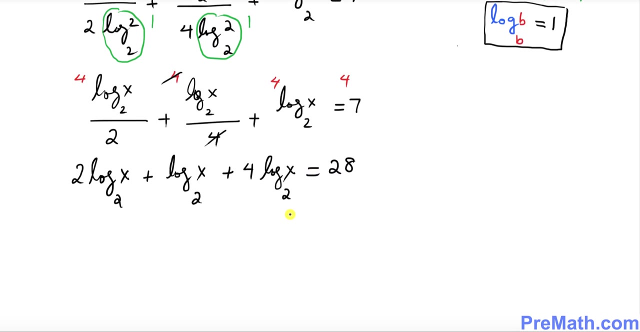 gone. so we ended up: log of x with the base. to here this become plus 4. log of x with the base 2, equal to 4 times 7, becomes 228. so far, so good. so let's go ahead. and so this is how much. this is 2. log x, x, base 2, and this is: 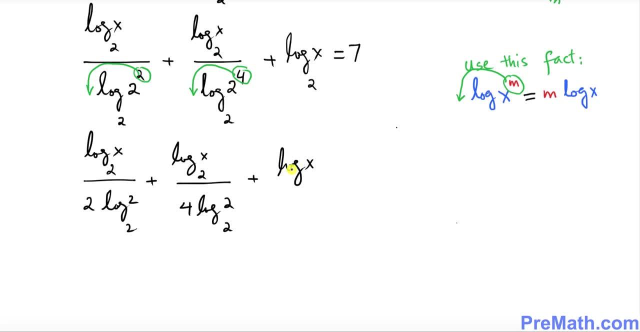 log of x, with the base 2 equal to 7. so next thing now I want you to just focus on this part. over here they have the, the base and the import. that's called. so, according to this fact, this turns out to be this: log of 2, with the base 2 turns out to be 1. 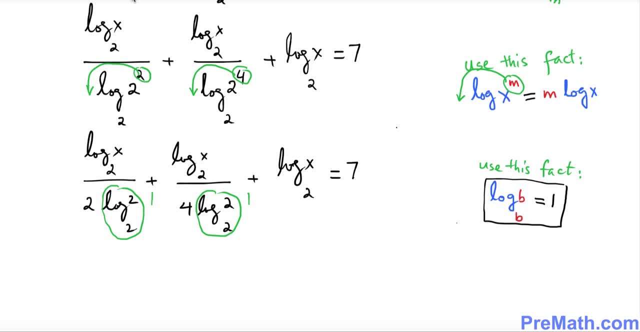 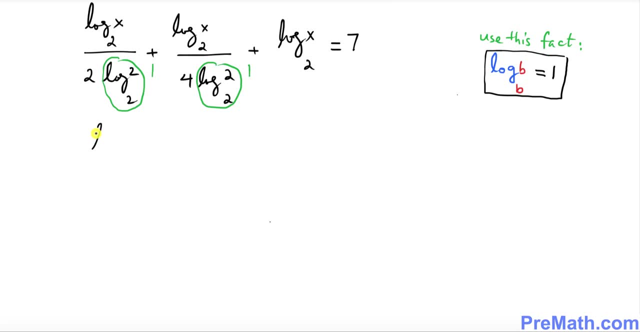 this is 1 and this is 1 as well, so our this problem could be more simplified, as you can see. log of x with the base 2 over 2 times 1, because this is 1, so this is simply 2 plus log of x with. 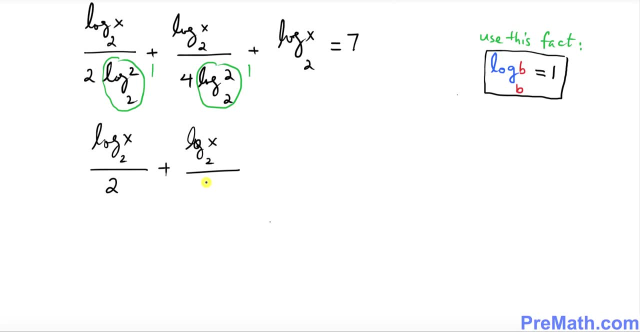 the base 2 divided by 4 times 1, 4 plus. now we have a log of x with a base 2 equal to 7. so we have these fractions over here. we want to remove them. in order to remove them, the best thing to do is I want you to multiply by the. 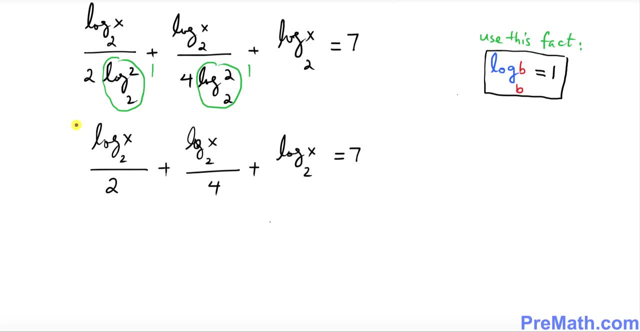 the biggest number over here at the bottom is 4, so I'm going to multiply by 4 across the board. okay, so once you do that one. so this 2 and 4 reduces to 2 times log of x with a base 2 plus this 4, and this 4 is gone. so we ended up log of x with a base 2 here. this become plus. 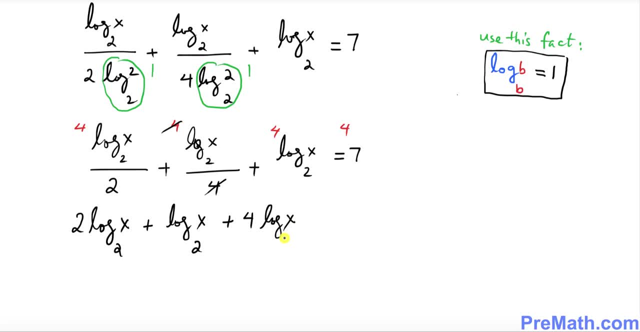 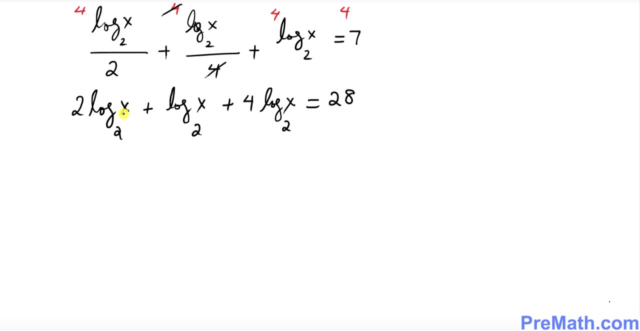 4 log of x. with a base 2 equal to 4 times 7 becomes 28. so far, so good. so let's go ahead. and so this is how much. this is 2 log x, x base 2 and this is a 1 log x base 2. and this is 4 log of x base. 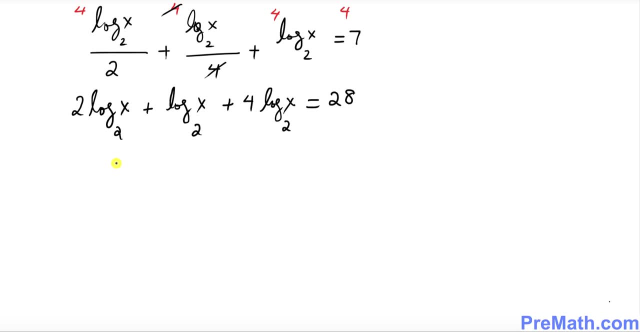 2 and you add them, 2 plus 1 plus 4 makes 7 log of x with a base 2 equals to 28. we want to isolate log, so I'm going to divide both side by 7 once you do that one. so we simply this: 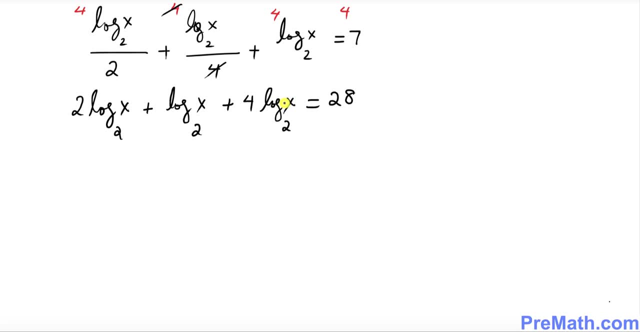 a 1 log x base 2 and this is 4 log of x base 2 and you add them, 2 plus 1 plus 4 makes 7 log of x with a base 2 equals to 28. we want to isolate log, so i'm going to divide both side by 7 once. 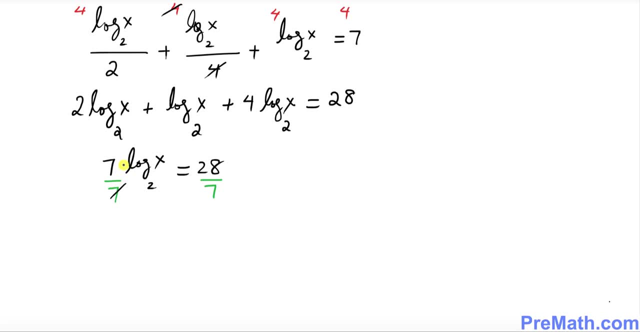 you do that one, so we simply this is gone. so log of x with a base 2 turns out to be 4 and finally, we're going to use this fact. we want to convert from logarithmic form to an exponential form, so this equation is going to look like: x equals to 2 power 4. so that means x equal to power 4 is. 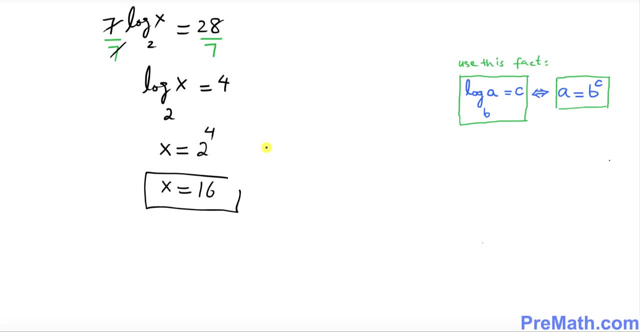 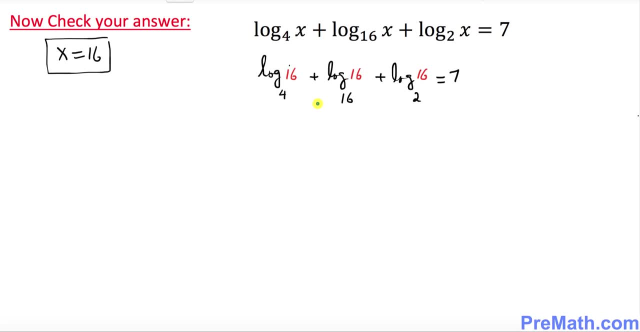 and the next step is: i want to tweak it. i want to manipulate a little bit 16. over here, you see this 16. want to manipulate a little bit 16. over here, you see this: 16. i can write this 16 as 2, 4 power 2, and here, this 16, i can write 2 power 4. so that's what i'm going. 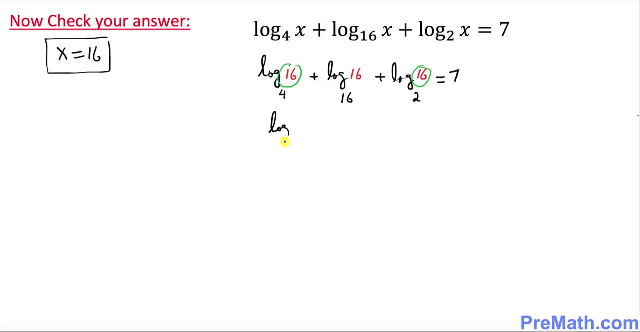 to do right now. i'm going to put down log of base 4. i can write 4 power 2. i'm going to leave this one same. there's a reason i'll tell you in a minute and plus this one, i can write base 2. 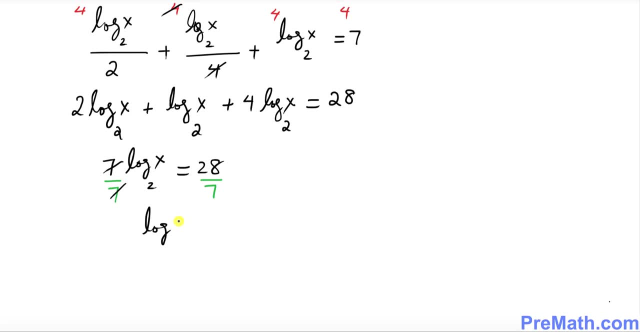 is gone. so log of x with a base 2 turns out to be 4. and finally, we're going to use this fact. we want to convert from logarithmic form to an exponential form. so this equation is going to look like: x equals to 2 power 4. so that means x equal to power 4 is 16, and that is our solution. and now 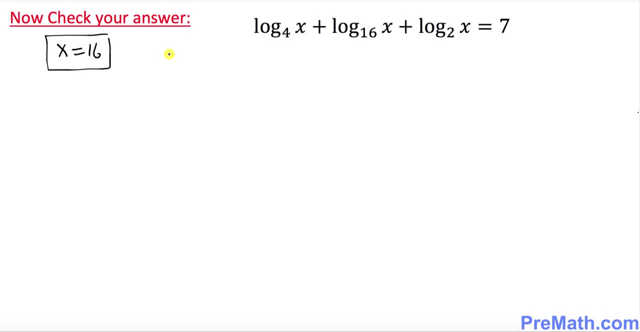 finally, we want to check our answer for any extraneous solution. so wherever you see x, replace it by 16. so what I did is: wherever you see x, I replace it by 16. and the next step is I want to tweak it, I want to manipulate a little bit 16 over here. you see this 16. i can write this 16 as 2, 4, power 2. 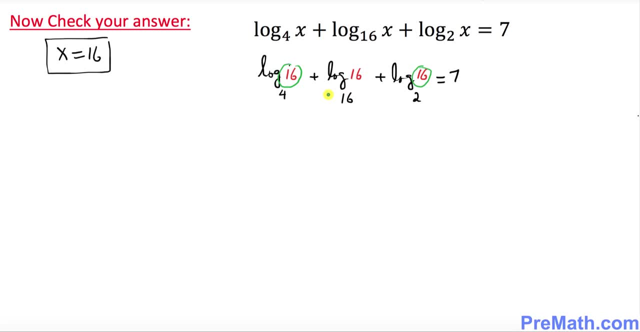 and here this 16. i can write 2 power 4. so that's what i'm going to do right now. i'm going to put down log of base 4. i can write 4 power 2. i'm going to leave this one same. there's a reason. 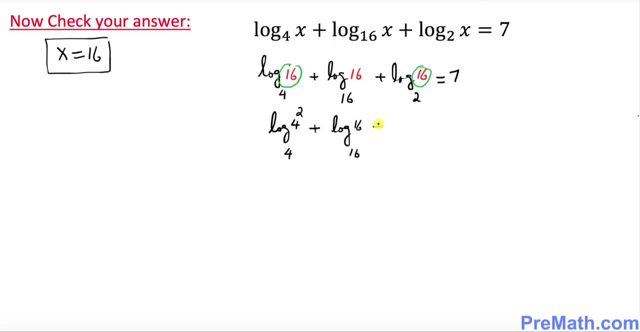 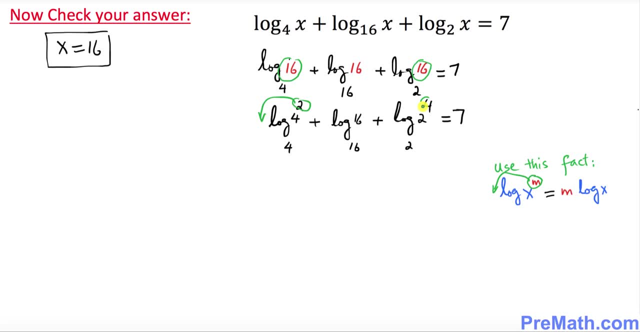 exponent this can move up to the front and this exponent moves up to the front as well. So we simply got 2 outside log of 4 with a base 4, plus log of 16 with a base 16.. Likewise, this 4 moves.